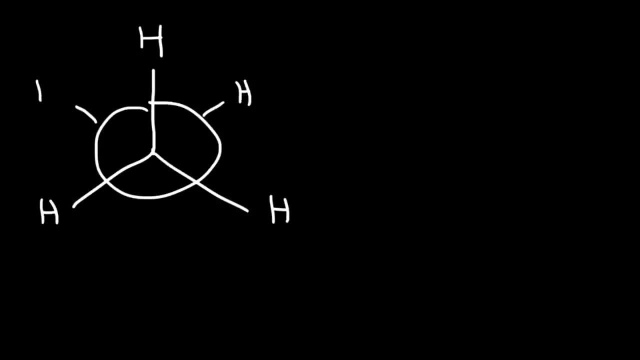 draw it like this. So this is the staggered conformation of ethane, Or you can draw the eclipse conformation. Which one do you think is more stable, The staggered conformation or the eclipse conformation? The hydrogens in the 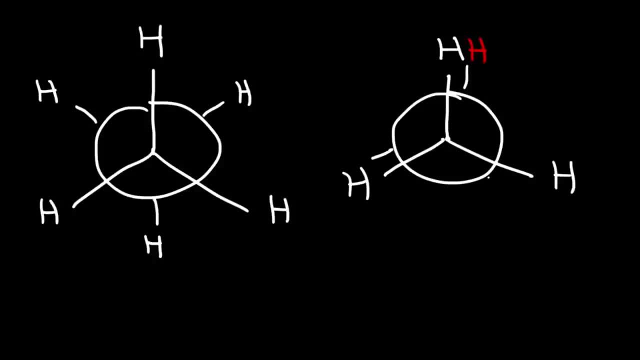 back. I'm going to draw it in red. You need to understand that the staggered conformation is more stable than the eclipsed, And the reason for that is this interaction: where the hydrogens are eclipsing each other, there's torsional strain, And so this conformation is going to be higher in 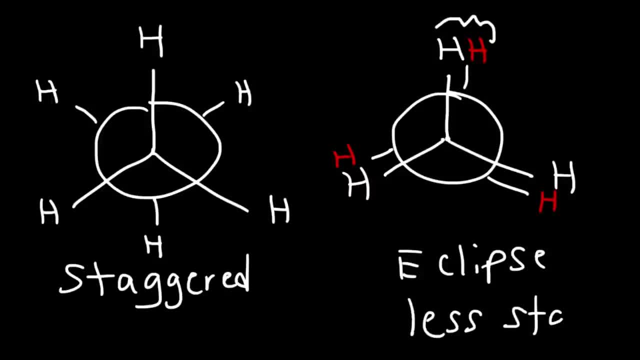 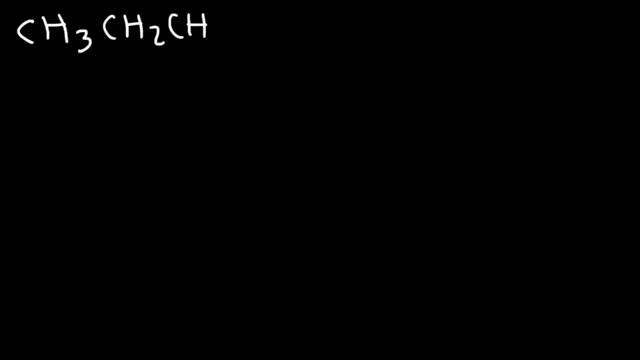 energy. So this is the less stable conformation, and on the left we have the more stable, staggered conformation. Now let's move on to our next example. So let's draw the Newman projection of butane along the C2-C3 bond. 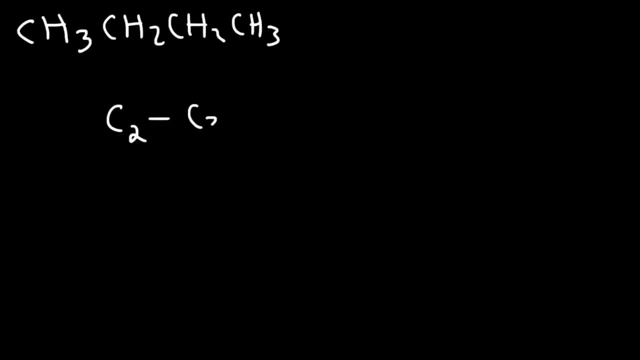 So first let's draw carbon 2 and carbon 3.. Now, attached to carbon 2, which is this carbon right here, it has a methyl group on the left and it's a CH2, so it has two other hydrogen atoms attached to it. 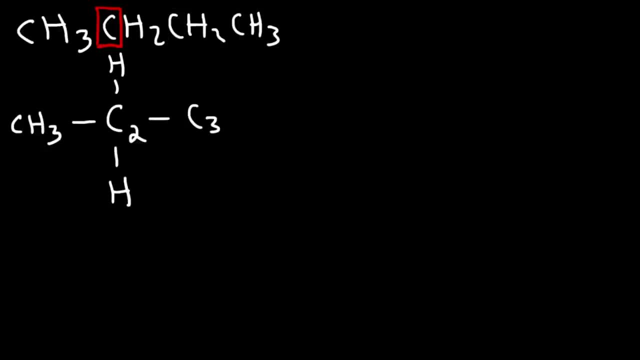 Now carbon 3, which is this carbon? I'm going to highlight that one in blue. it's also attached to two hydrogen atoms and a methyl group, And so we need to draw everything around this C2-C3 bond. So now let's draw a Newman projection. 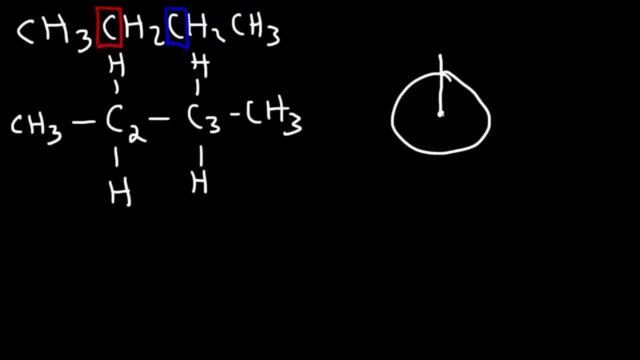 So I'm going to draw a smaller version this time. So this is going to be carbon 2, which I'm going to highlight in red, this red dot. So carbon 2 is in the front and carbon 2 has a hydrogen, another hydrogen. 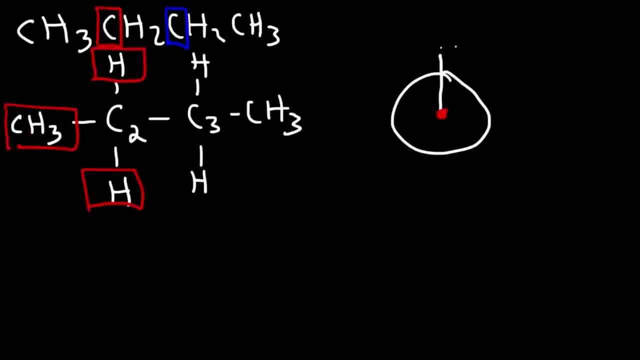 and a methyl. I'm going to place the first methyl group at the top and then the other two hydrogens. Now carbon 3,, which is in the back. it also has two hydrogens and one methyl group. So I'm going to place this methyl group at the bottom and these hydrogens on this side. 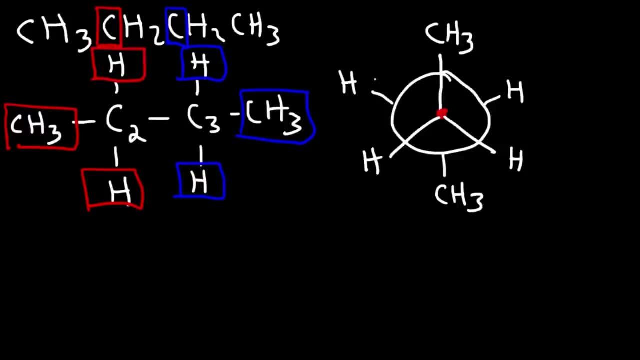 So this is a staggered conformation, but it has a specific name, called an anti-conformation. It is the most stable of the four Newman projections of butane. The reason for that is because the methyl groups are so far apart. You want to keep them as far apart as possible. 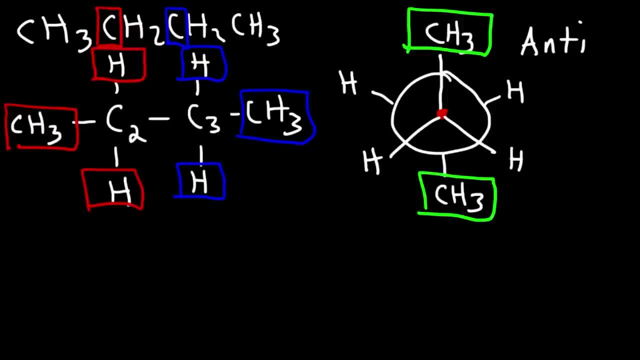 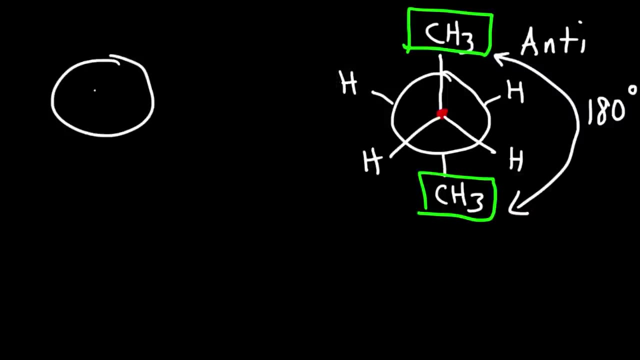 And so this is the anti-conformation of butane. The dihedral angle between these two methyl groups is 180.. Now let's draw the other conformations of butane. So I'm going to keep the first methyl group at the top. 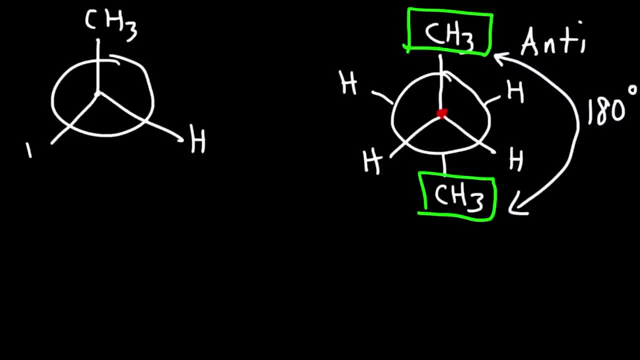 I'm not going to change that position. Now, the second methyl group: we can put it right here, and so the other hydrogens will be around it, And so, as you can see, we don't have the eclipsed conformation yet. 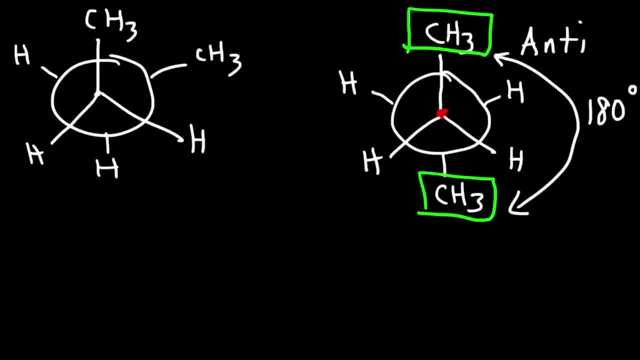 This is still another type of staggered conformation. However, this particular conformation is known as the Gauch conformation or the Gauch conformation, And the dihedral angle between the two methyl groups is 60 degrees. Now there is some steric strain when the methyl groups are close to each other. 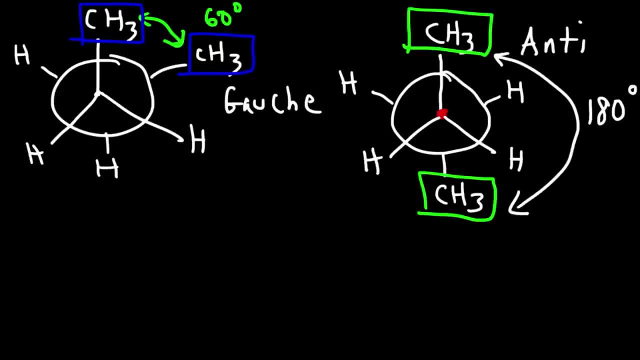 And so whenever you have this Gauch interaction, when they're 60 degrees apart, you're going to have this steric interaction. So therefore, the Gauch conformation is less stable than the anti-conformation. This is going to be number one, meaning it's the most stable. 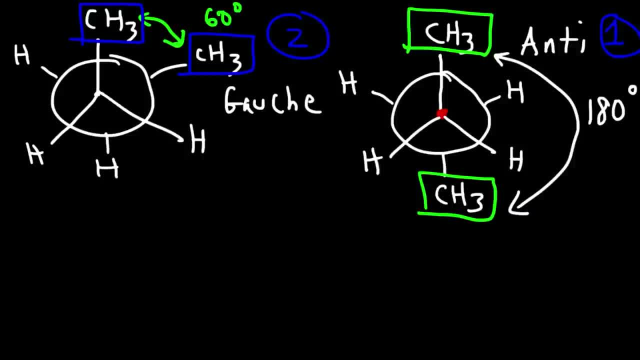 This is number two. It's the second, It's the most stable. Now there's two types of eclipsed conformation that we can draw. The first one, which I'm going to show in red: the hydrogens. a hydrogen eclipsed- the. 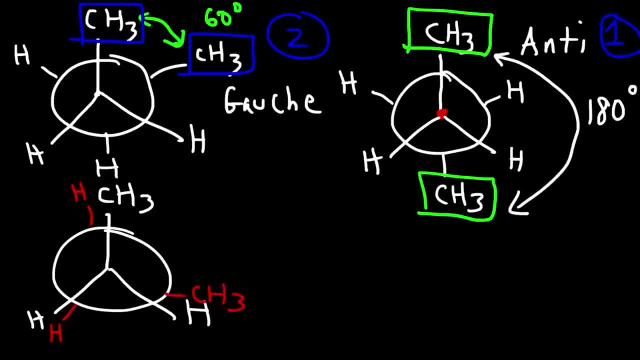 methyl group and we have this methyl group eclipsed in the hydrogen. So this is the third most stable conformation And then, in the least stable conformation, the two methyl groups eclipse each other. Now think of the sun or the moon eclipsing the sun. 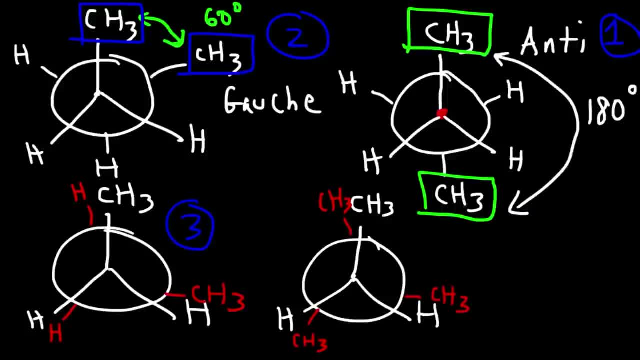 The moon could completely block out the sun, and that's what's happening here. The white methyl group is eclipsing the red methyl group, So technically you should not be able to see the red methyl group. It should be like directly behind the white methyl group. 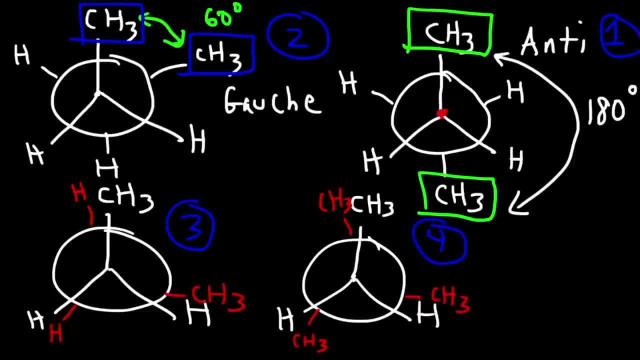 So this is called totally eclipse. It's the least stable of the four conformations of butane. Now let's go over the angles for each one. So, going back to the Gauch conformation, if you notice the angles between the methyl groups, 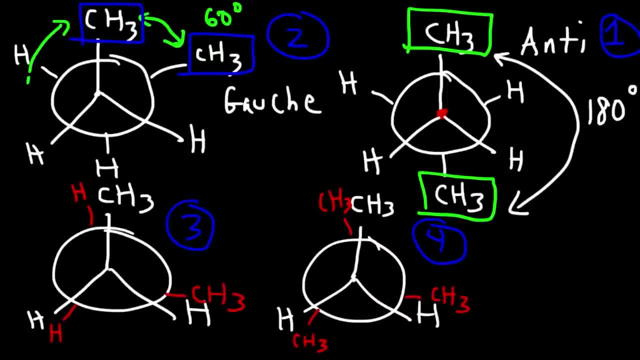 is 60 degrees, Or if you go in the other direction, it's 300. So there's two angles that correspond. So this conformation, 60 and 300.. Now for the eclipse, conformation number three: notice that the methyls are 120 degrees apart. 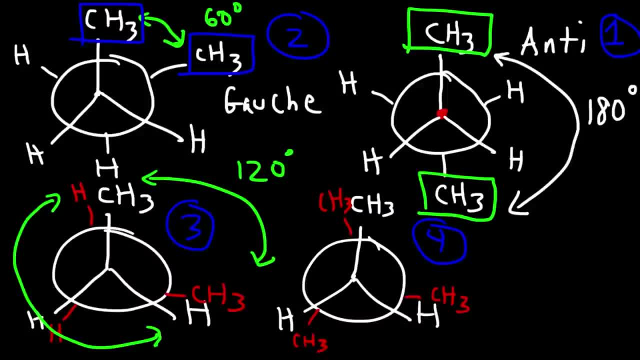 Or, if you count it in the other direction, they're 240 degrees apart, Because 240 plus 120 adds up to 360.. And for the last one it's zero degrees apart. Zero degrees and 360, they're the same. 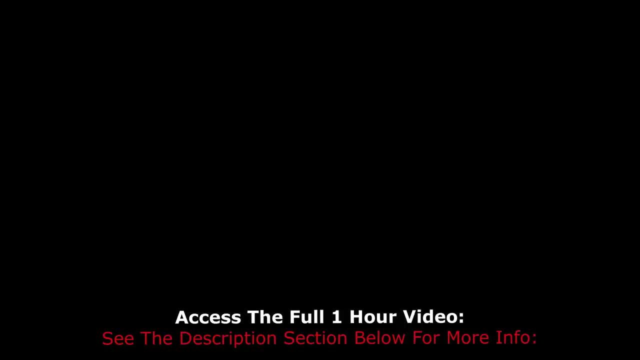 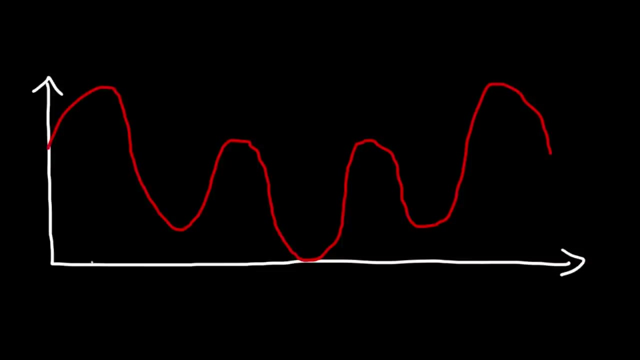 Now, the reason why I mention that is because when drawing the potential energy diagram, you can see how it relates to each other. So this angle is the zero degree angle. Here. this is going to be 60. And then 120.. And then this is 180.. 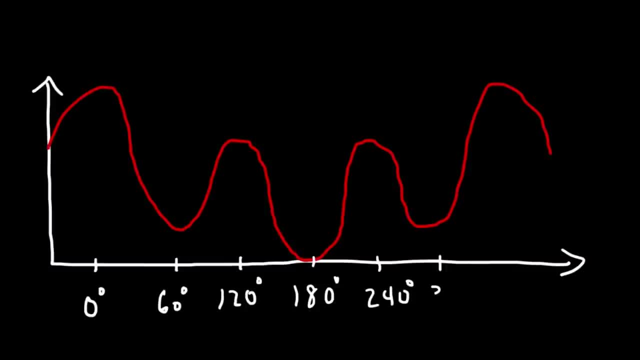 240.. And then 300. And then back to 360.. So the anti-conformation is the one with the lowest energy. All right, So on the y-axis we have potential energy. On the x-axis it's the dihedral angle. 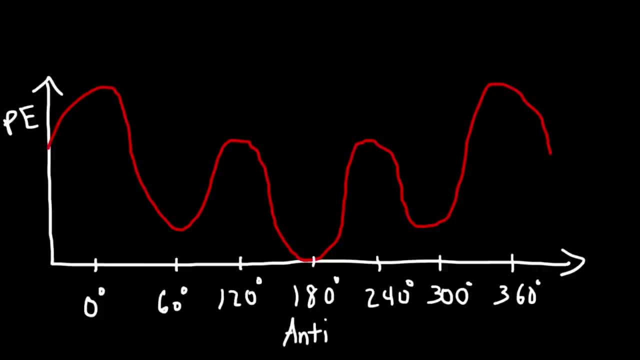 So recall that the anti-conformation, which we said was the most stable, it had a dihedral angle of 180.. And so it has the lowest energy. So this was structure number one, the most stable. The second one was number two. 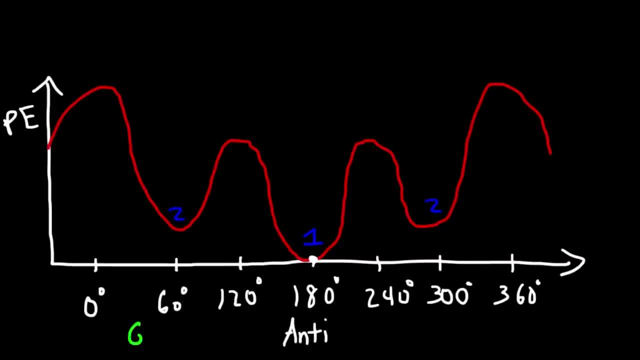 And number two was the Gauch interaction And it had a dihedral angle of 60 and 300. Which we saw on the previous page. And then structure number three was the eclipse conformation, which I'll write E for eclipse. 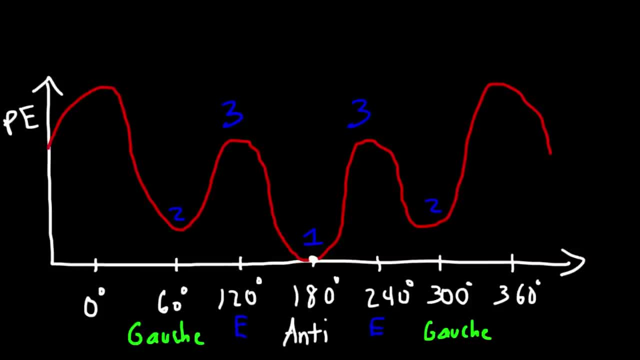 And it had two angles- 120 and 240, which we see here. And then structure number four. that was the least stable, So it has the highest potential energy, And it had a dihedral angle of zero. So that was the total eclipse structure. 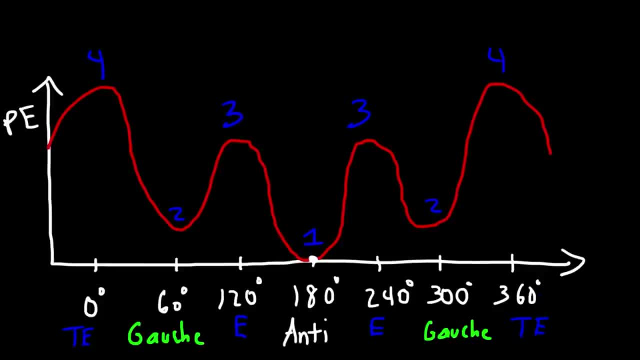 Or total eclipse, rather And zero and 360.. 360 are the same, So you could see where they're located on this potential energy diagram. So as the potential energy increases, the stability of the molecule decreases. Highly stable molecules have low potential energy. 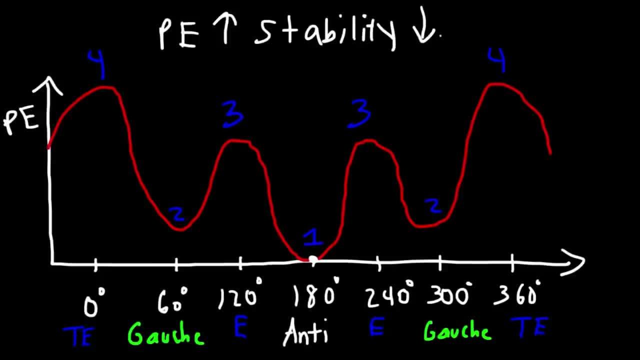 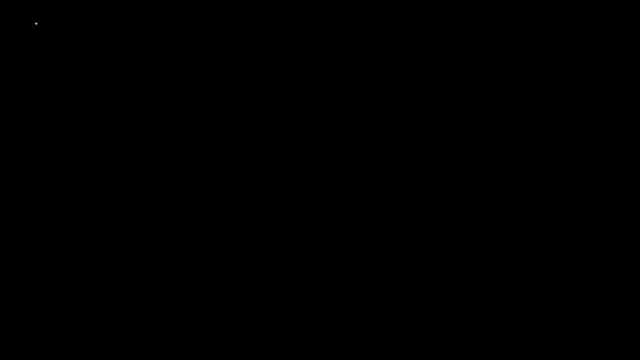 And unstable molecules have high potential energy. So that's it for butane. Let's draw the Newman projection of, let's say, 2, 3.. And that's it, 3-dimethylpentane. So feel free to pause the video and try that. 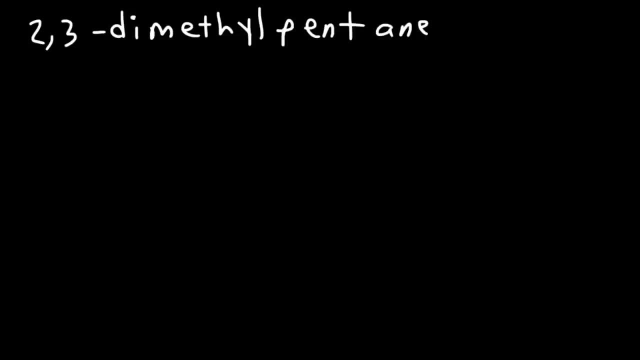 And identify which of those Newman projections- this could be many- which one is the most stable out of the ones you can draw. So first let's draw a line structure. So here we have pentane, And then we have a methyl and carbon 2 and 3.. 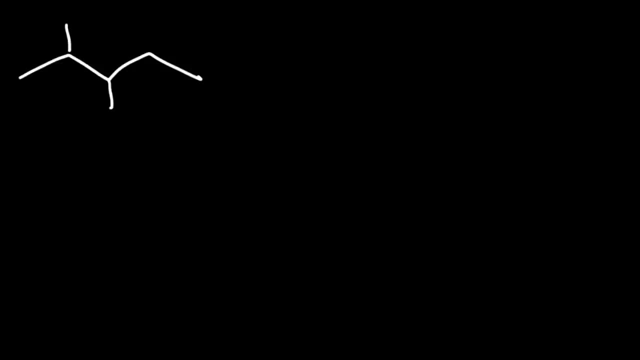 And also I need to specify that we need to draw the Newman projection along the C2-C3 bond. I don't know what you have drawn, So this is CH3.. And then we have a CH And then another CH3. 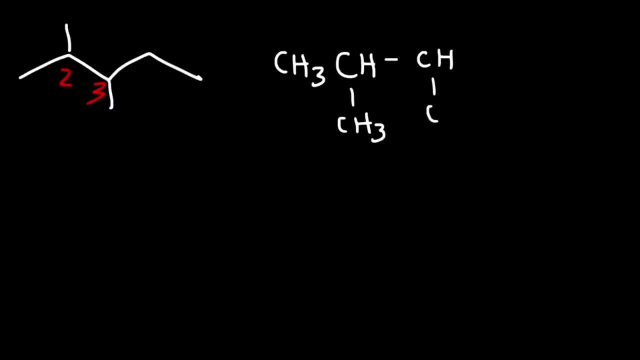 And then it's a CH, CH3, CH2, CH3.. So this is carbon 2.. And this is carbon 3.. So carbon 2 has 2 methyl groups. Now what does that mean groups? and it has a hydrogen. 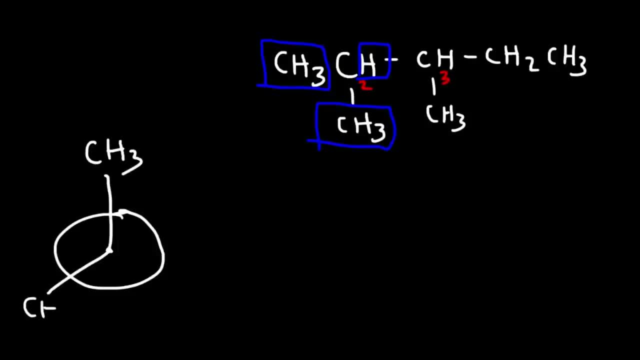 So here's the first methyl group on carbon 2, here's the second one, and then here is the hydrogen. Now for carbon 3, it too has a hydrogen, a methyl group, but it also has an ethyl group. So let's put that in the back. 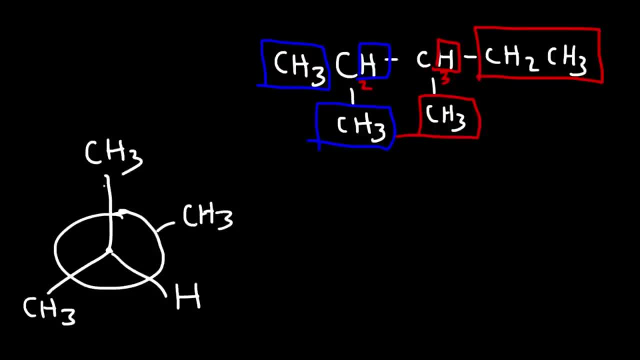 So here is the methyl group, here's the hydrogen and here is the ethyl group. So what other Newman projections can we draw of this molecule of 2,3-dimethylpentane? So this is carbon 1, carbon 2 has a methyl group, carbon 3 is behind it, which also has 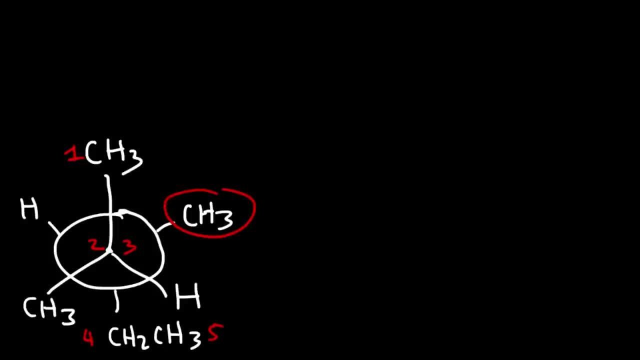 a methyl group. So this is carbon 1, carbon 2 has a methyl group, carbon 3 is behind it, which also has a methyl group, And then here's 4 and 5. So we have a total of 7 carbon atoms. 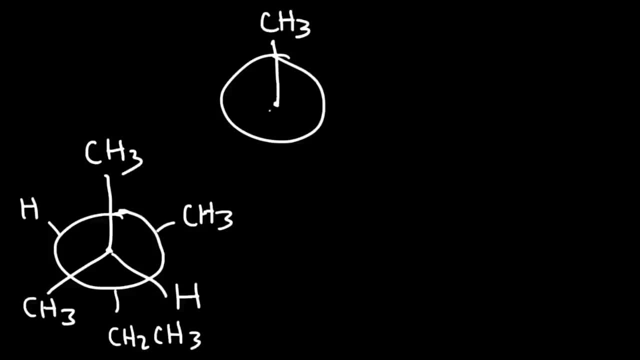 So let's redraw the stuff around carbon 2, the two methyl groups with the hydrogen. Now, another staggered confirmation that we can draw is we can put this ethyl group where this methyl group is, And so that's going to give us 2.5-dimethylpentane. 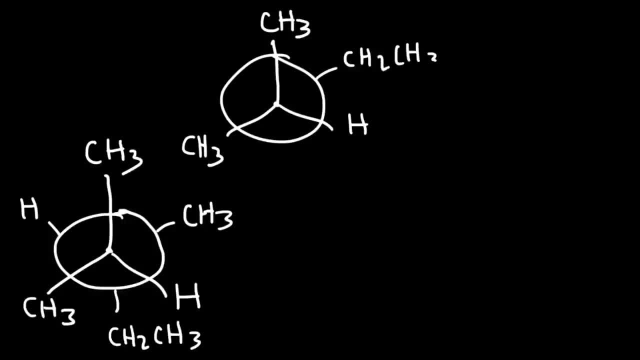 And then here's 4 and 5.. Now are these two staggered confirmations that I'm drawing right now or the two that I have on the board? are these two the same or are they different? Notice that they're equivalent to each other, because here we have a Gauch interaction. 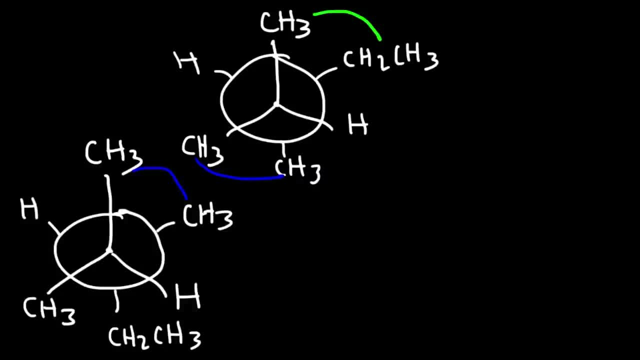 the same on this side and there's another Gauch interaction between the methyl and the ethyl. So, as you can see, these two structures are identical. however, we could create a different structure If we place a methyl group here and then the ethyl group here. 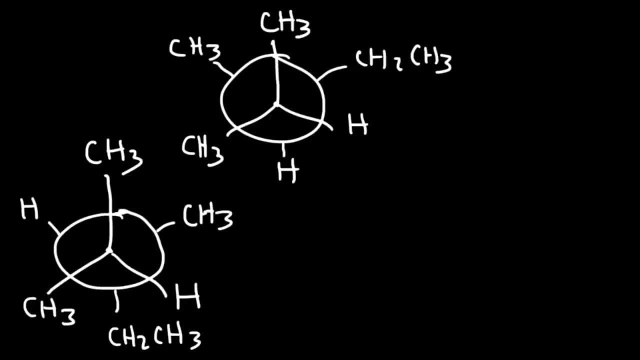 So that's a different, staggered confirmation. In our original structure we had one methyl-methyl-Gauch interaction. In the new structure we have two methyl-methyl-Gauch interactions, And in the old structure we have two methyl-methyl-Gauch interactions. 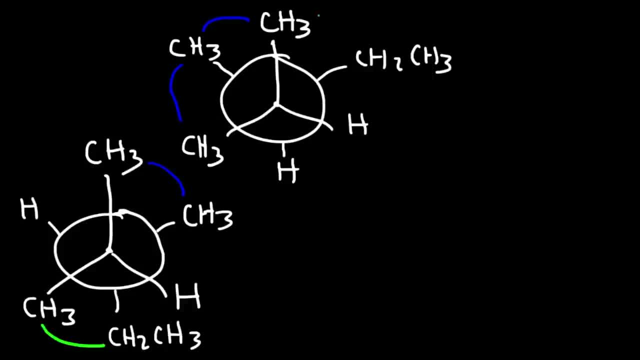 structure. we had one methyl ethyl gout interaction, but a new structure. we have just one methyl ethyl gout interaction. so in this new structure we have a total of three gout interactions. in the original one we have two. so this structure here is less stable, and then this one. now let's see if we can draw. 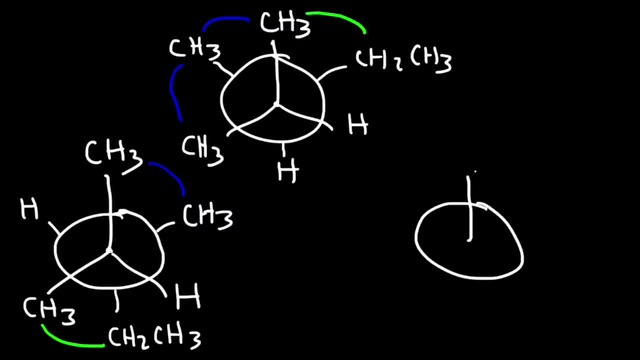 another staggered Newman projection, because I think we can, and we can do so if we put the ethyl between the two methyl groups and let's put the methyl here. so this time we only have one methyl methyl gout interaction, but now we have two methyl ethyls gout interactions. and because ethyl is. 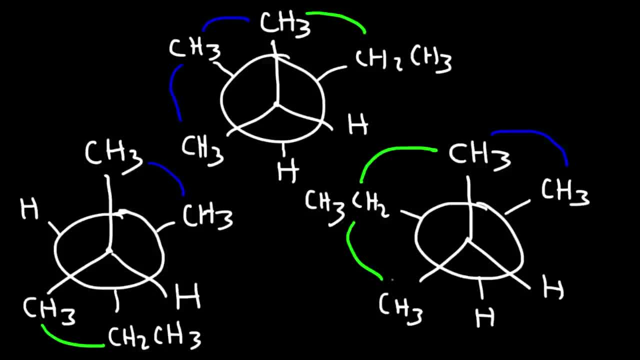 bulkier than methyl. it stands to reason that an ethyl methyl gout interaction has more energy than a methyl methyl gout interaction. so, therefore, this is going to be number one, the most stable, staggered confirmation that we can draw. this is going to be number two and this is going 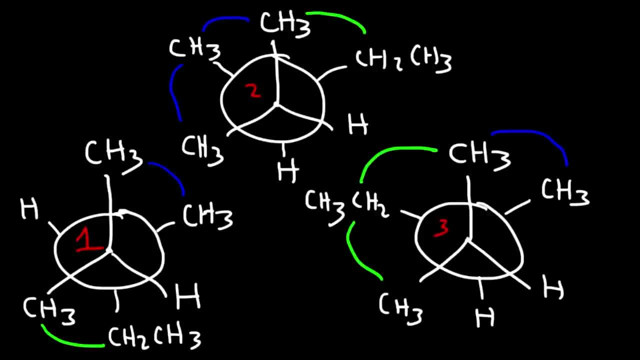 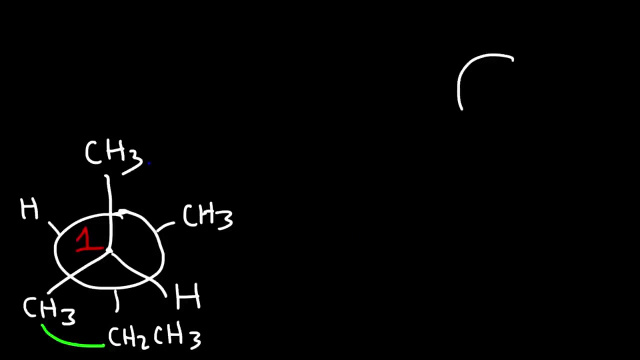 to be number three, the least stable of all the staggered confirmations that we can draw, based on the idea that an ethyl methyl interaction has more steric strain than a methyl methyl interaction. now let's draw the Eclipse confirmations. so let's start with this part first, and I'm going to begin by eclipsing the. 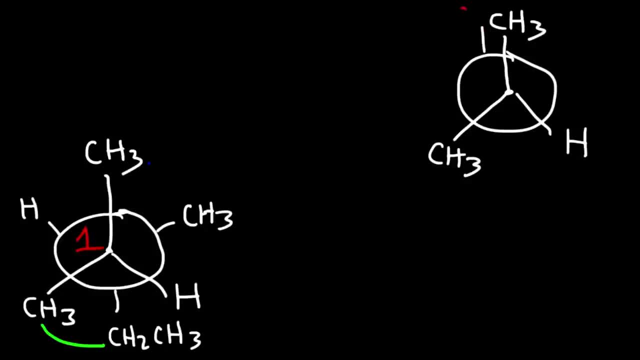 methyl groups together, let's make this an ethyl group, and then this is going to be the other hydrogen. now let's try the next structure. so here we have an eight H H Eclipse interaction. so now let's put a methyl group next to the hydrogen. so 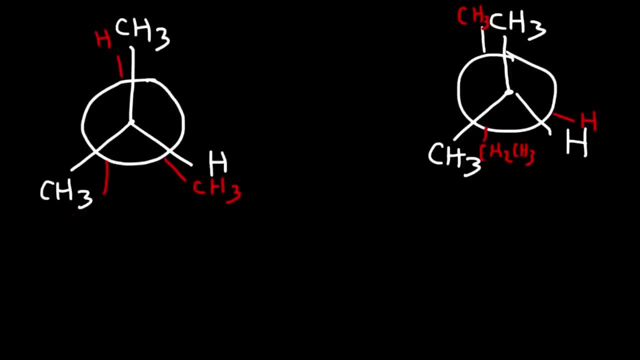 that's going to be different. let's keep the ethyl group on this side. if we put the ethyl group here is the same as putting it here, because the two methyl groups are the same. now the only other different structure that we can draw is we can put the ethyl group next. 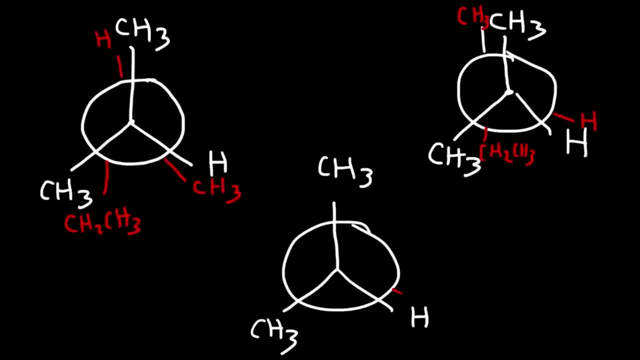 to the hydrogen. that will be different than the first two, and then one hydrogen has to be with one of the other methyl groups, and the other methyl group has to be there too. now I'm going to leave it up to you to rank the stability of these three. 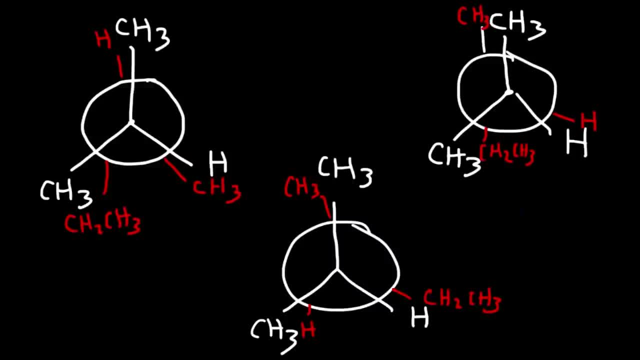 eclipse confirmations. but just to get you started, it's good to know that whenever you have two hydrogen atoms eclipsed to each other, the torsional strain energy value is about four kilojoules per mole, and when the hydrogen eclipses a methyl group, it's 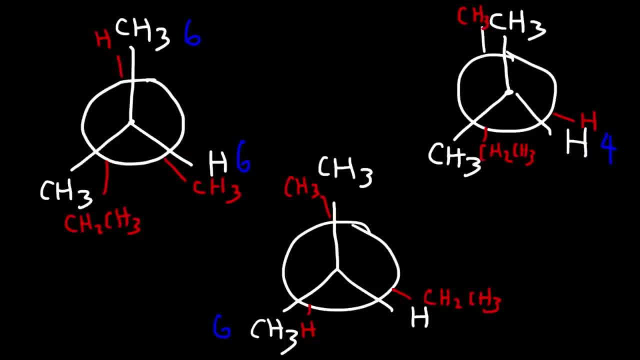 about six kilojoules per mole. whenever you have two methyl groups eclipsing each other, the energy value is 11. so we have enough information to compare these two molecules because these two interactions between a methyl and ethyl group. they're the same, so we don't have to take that into account. so for the two remaining, 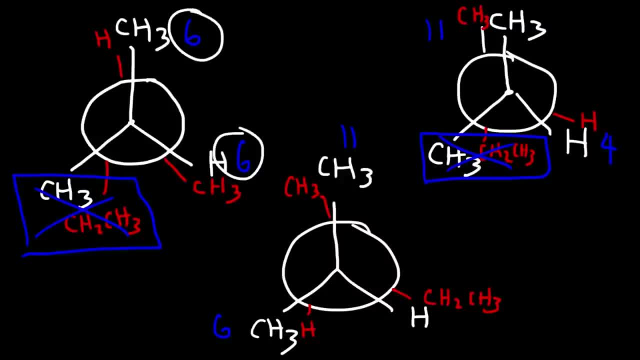 groups. this has a total energy profile of 12 and for this one it's 15, not taking the ethyl methyl interaction into account. so because the structure on the right has a higher potential energy value, we could say it's less stable than the structure on the left. so the structure on the left is. 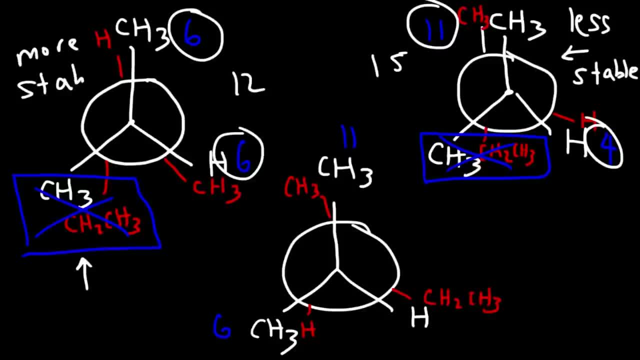 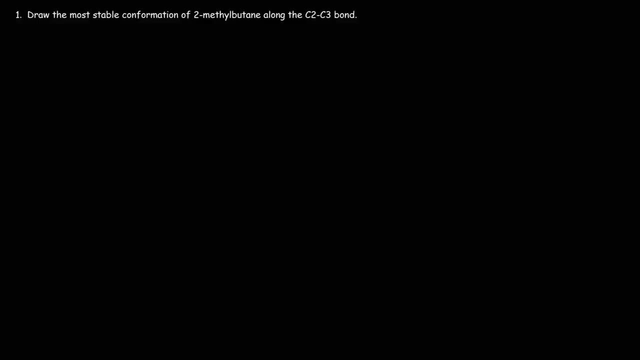 going to be more stable. now I'll leave it up to you to do research to determine how this molecule compares to the other two. so you need to determine the energy value between a methyl and the hydrogen- I mean a ethyl and a hydrogen, and also ethyl and a methyl- in order to answer that question. now let's work on some. 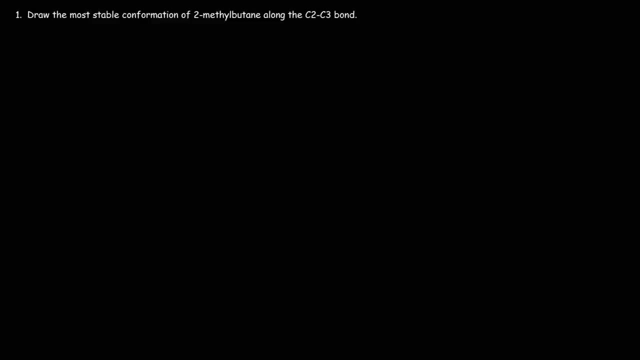 practice examples. number one: draw the most stable confirmation of two methyl butane along the c2c3 bond. feel free to pause the video and try this example. so let's start with the line structure of two methyl butane. so first we're going to draw butane and then we have a methyl group on carbon two. 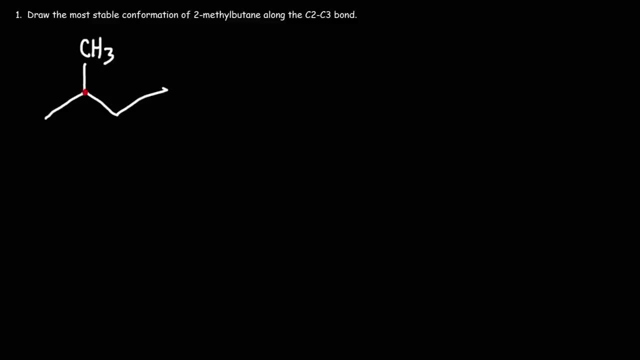 so this is carbon two and this is carbon three. now let's draw everything else that's attached to those two carbons. so in carbon two we have another methyl group and is a hydrogen. keep in mind carbon can only form four bonds. and carbon three has a methyl group attached to it, but it has two hydrogens. so let's. 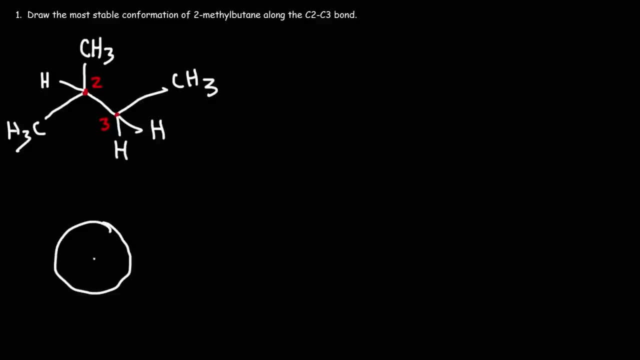 draw our first new projection. so we're going to have carbon two. in front we have our first methyl group and then we have another methyl group to the left and then the hydrogen. so here are the three things that we've added. so now to the back, carbon. 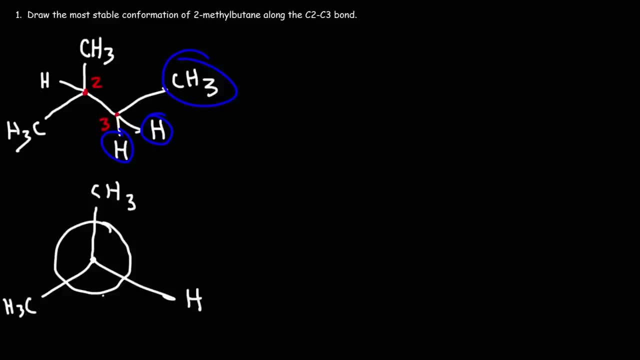 or carbon three. we're going to add these three groups, so I'm going to start by putting the methyl at the bottom. any other two hydrogen atoms here. so notice that in this particular confirmation of two methyl butane you only have one gauch interaction with an energy profiler of 3.8 kilojoules per mole. now 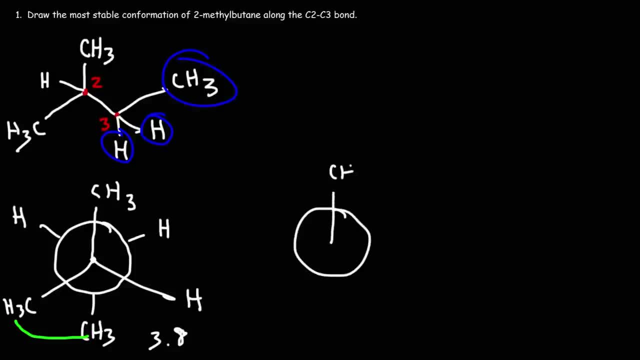 let's draw another one, let's see what other new and projections that we can draw so we can compare it to our first example. so the first three groups i'm going to keep the same. let's put this methyl group here and then we can place the other two hydrogen atoms. 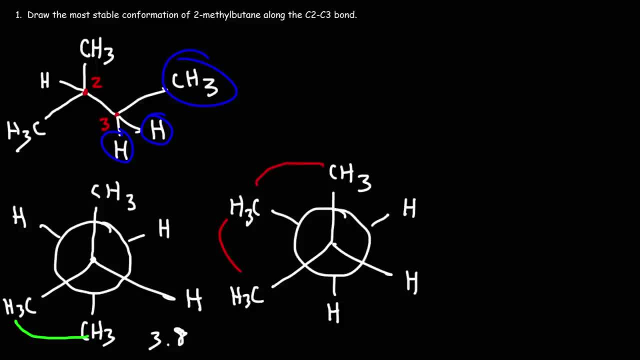 so notice that we have two gauch attractions. so the energy profile for this particular confirmation is going to be 3.8 plus three point eight. and the last Gaz celebrities are going to be three. widespreadKnuke and other hydrogenMA3s are going to be four, must be more. 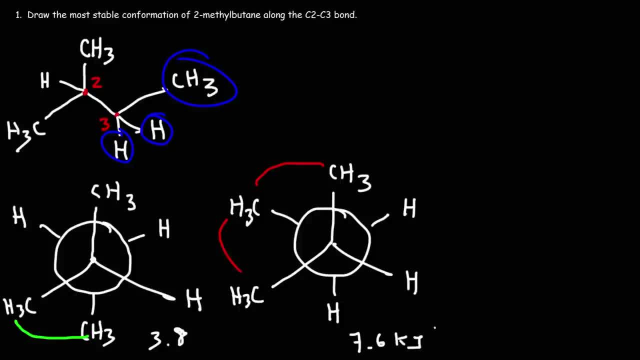 which is 7.6 kilojoules per mole. So far we've placed the methyl group in this position and in this one. Let's see what happens if we put it there. So if we put it towards the right, the other hydrogen atoms have to go in the other position. 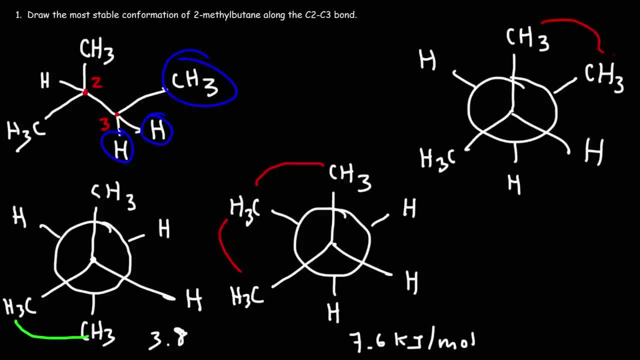 So we only have one Gauch interaction. In fact, these two conformations are the same. So those are all of the stable staggered conformations that we can draw. We know that the Eclipse conformations will be less stable, so we're not going to draw them. 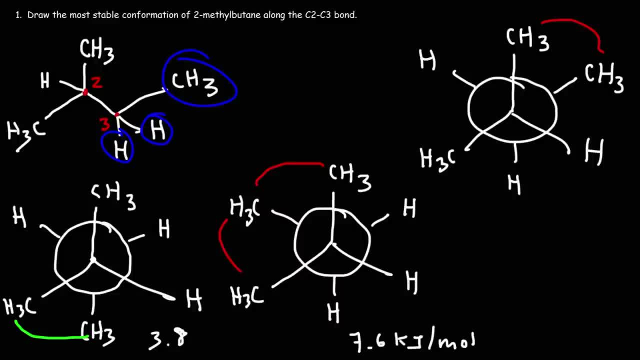 The one that is the most stable is the one with the lowest potential energy, So therefore, this particular conformation of 2-methylbutane is the most stable. So this is our answer, Number 2.. Consider the following conformations of butane: 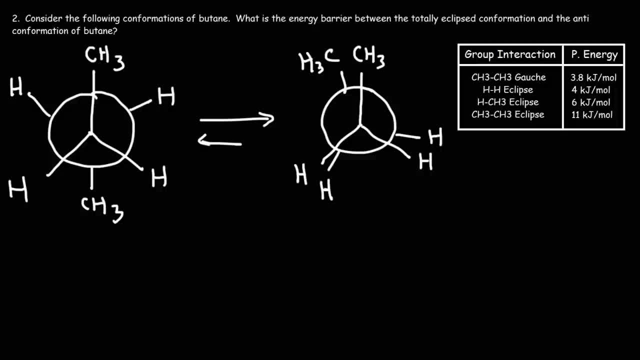 What is the energy barrier between the totally Eclipse conformation and the anti-conformation of butane? Now, the energy profile for the anti-conformation, which is on the left, is basically zero. We don't have any Gauch interactions and there's no staggered or. 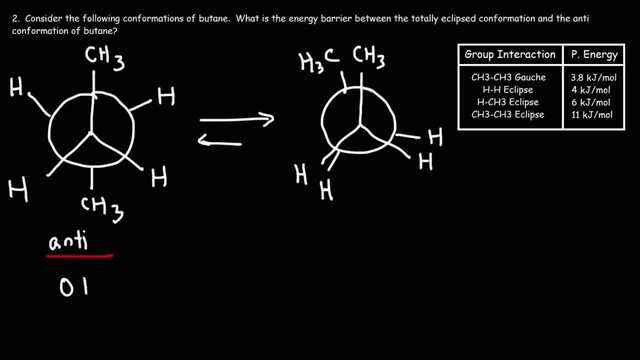 I mean there's no Eclipse interactions. So that's the energy profile. now, on the right, we have the totally Eclipse confirmation. so what's the energy profile for that, based using the the table on the right? the table on the right gives us the corresponding potential energy for each. 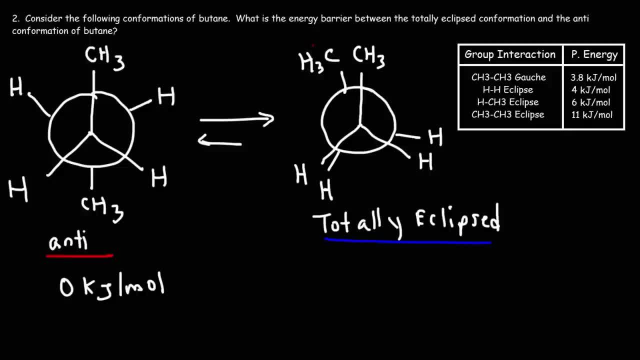 group interaction. so here we have two CH trees that are Eclipse to each other, so the energy value for that is 11. and then we have two hydrogen atoms that are Eclipse as well, so the energy for each is 4. so if we add 11 plus 4 plus 4,